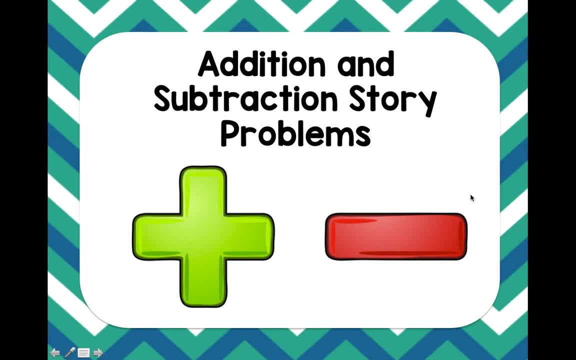 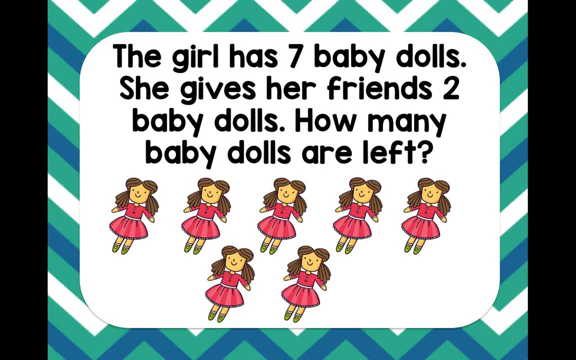 or a subtraction problem where we need to subtract with the minus sign. Are you ready? Okay, here's the story. The girl has seven baby dolls. She gives her friends two baby dolls. How many baby dolls are left? So let's listen to the story again. 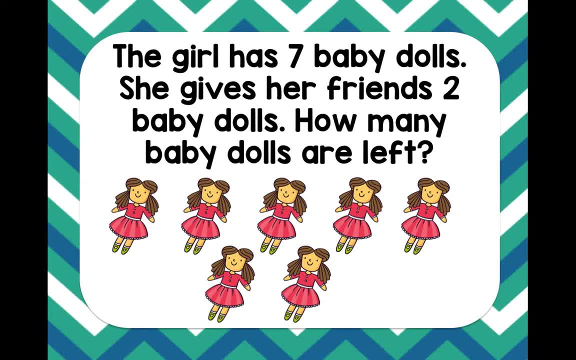 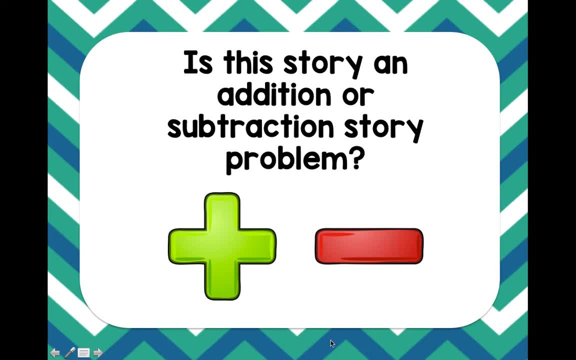 The girl has seven baby dolls and she gives her friends two baby dolls. Is this story an addition problem, where we use the plus sign, Or is it a subtraction problem, where we use the minus sign and we take away? It's a minus sign because she's giving her baby dolls away. 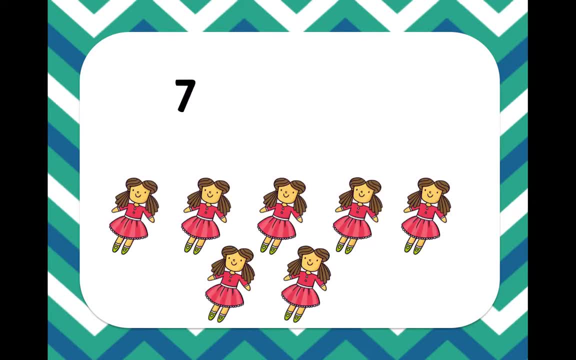 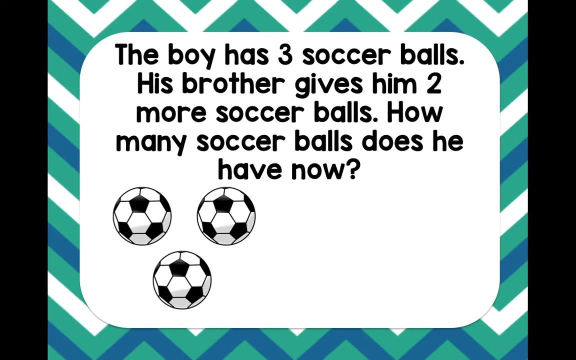 That means minus take away. So she has seven minus Two. take away the two baby dolls equals one, two, three, four, five. So seven minus two equals five. Here's another story: The boy has three soccer balls. 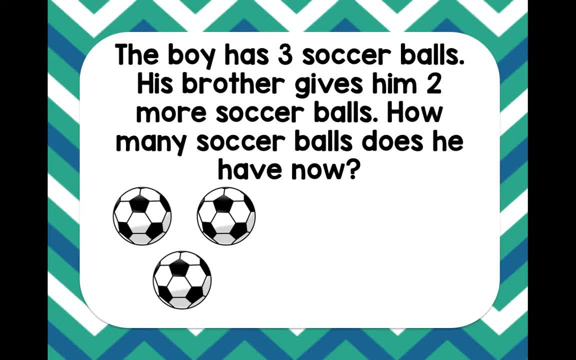 His brother gives him two more soccer balls. How many soccer balls does he have now? So we got to think: is this using the plus sign or the minus sign The boy has? The boy has three soccer balls and his brother gives him two more. 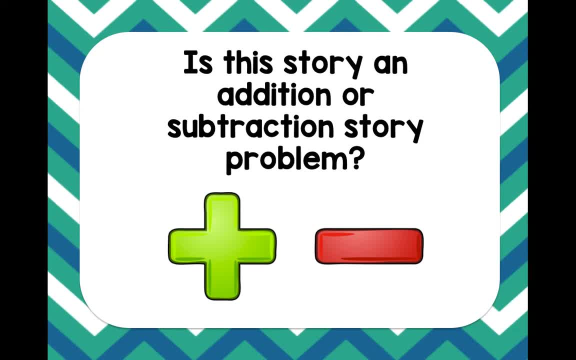 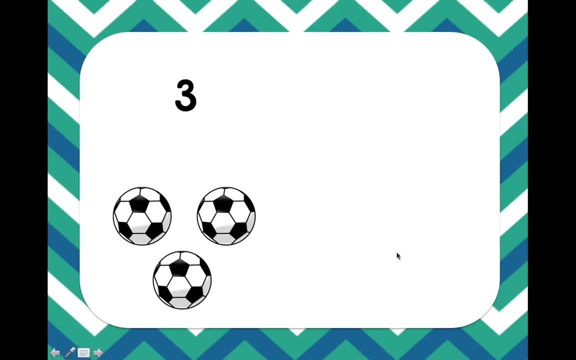 Is this an addition or subtraction problem? Is he getting more or is he taking away some soccer balls? He's getting more. So when we get more we add with the plus sign right. Plus that makes a bigger number. So he has three soccer balls plus two soccer balls equals one, two. 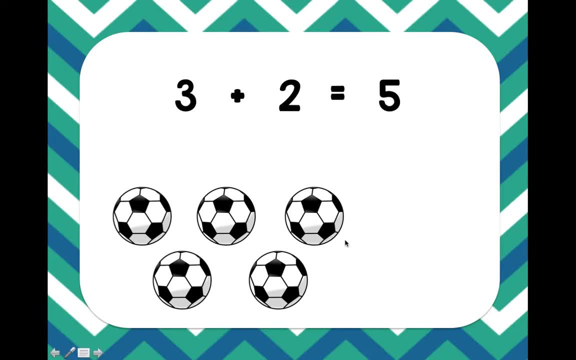 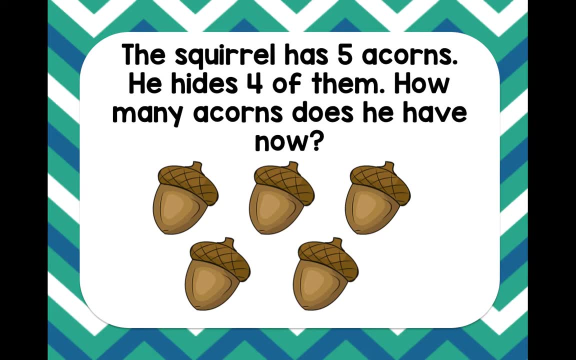 three, four, five. okay, So he has one, two, three, four, five soccer balls. now, All right, here's another story. The squirrel has five acorns. He hides four of them. How many acorns does he have now? 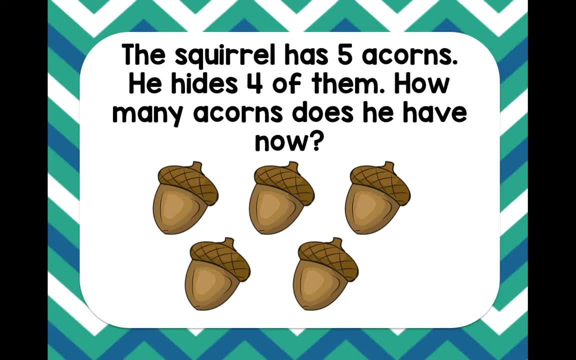 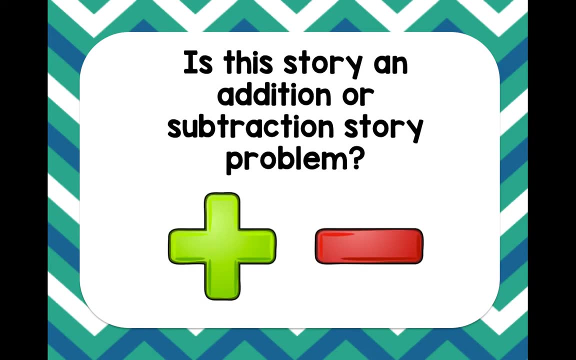 Is this an addition problem with a plus sign or a minus subtraction problem? Listen to the story again. The squirrel has five acorns, He hides four. He hides four of them. Is this a story, an addition or a subtraction story problem. 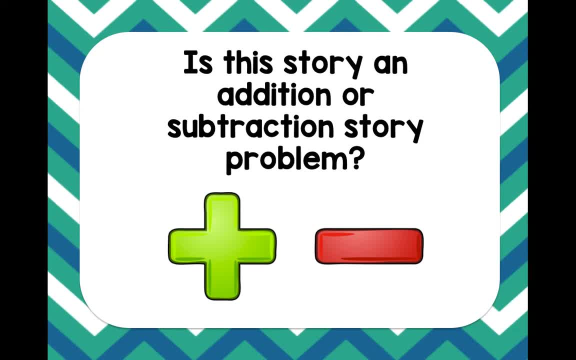 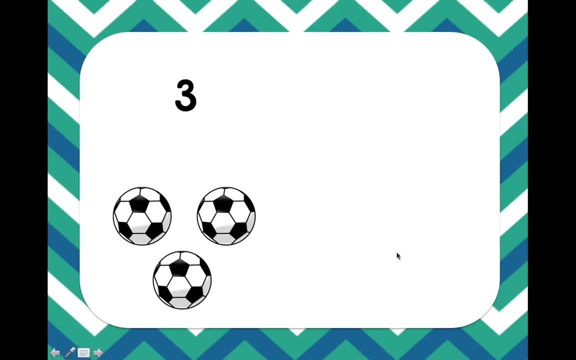 Is this an addition or subtraction problem? Is he getting more or is he taking away some soccer balls? He's getting more. So when we get more we add with the plus sign right. Plus that makes a bigger number. So he has three soccer balls plus two soccer balls equals one, two. 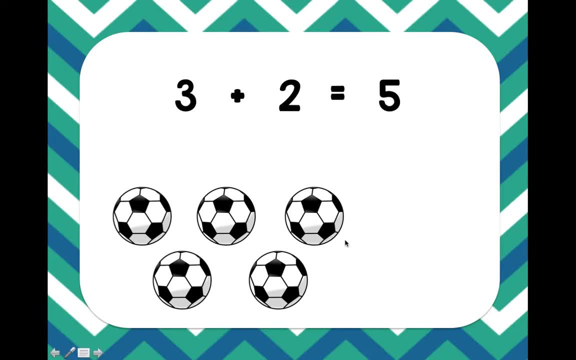 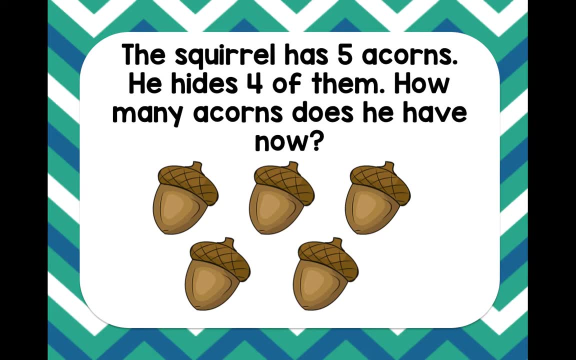 three, four, five. okay, So he has one, two, three, four, five soccer balls. now, All right, here's another story. The squirrel has five acorns. He hides four of them. How many acorns does he have now? 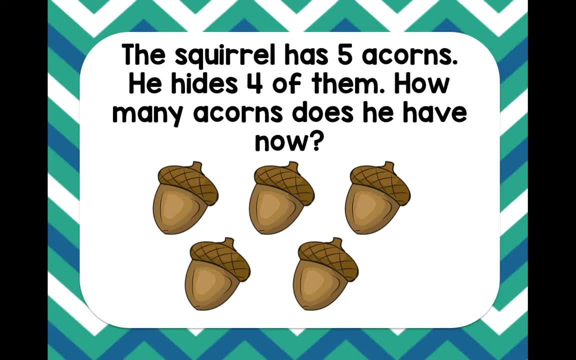 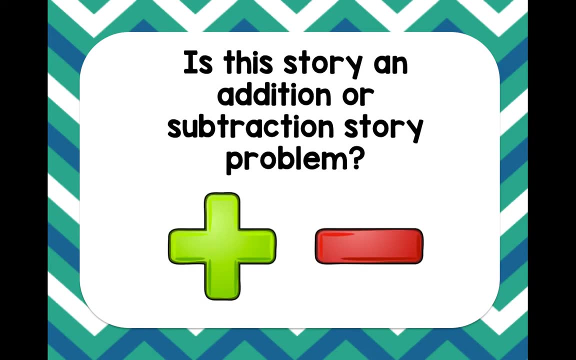 Is this an addition problem with a plus sign or a minus subtraction problem? Listen to the story again. The squirrel has five acorns, He hides four. He hides four of them. Is this a story, an addition or a subtraction story problem. 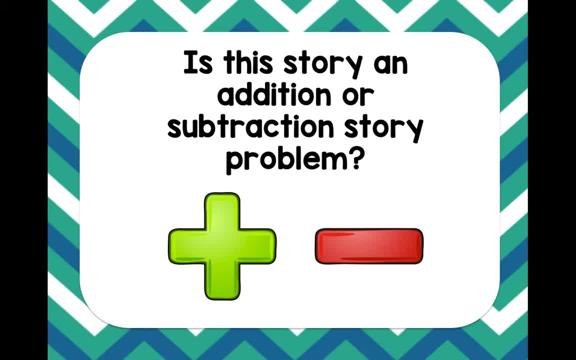 Is he getting more acorns or is he taking some acorns away? He's taking some acorns away, right, He's hiding them, So he's taking them away. That means the minus sign. So he has five acorns minus. how many does he hide? 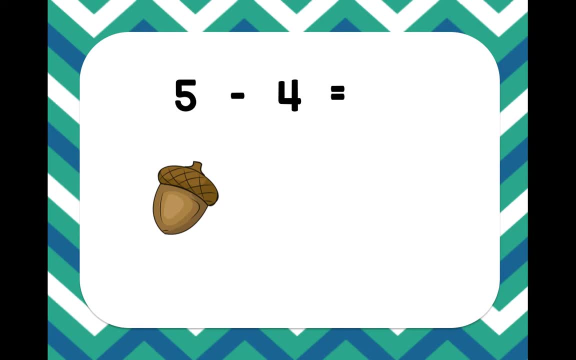 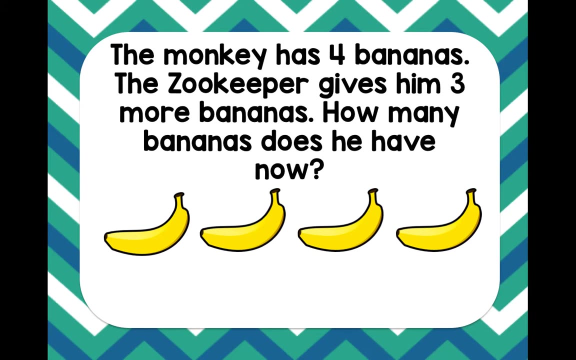 Four. One, two, three, four equals. how many does he have left to eat right now? One Good, The monkey has four bananas. The zookeeper gives him three more bananas. How many bananas does he have now? So the monkey has four and the zookeeper gives him three more. 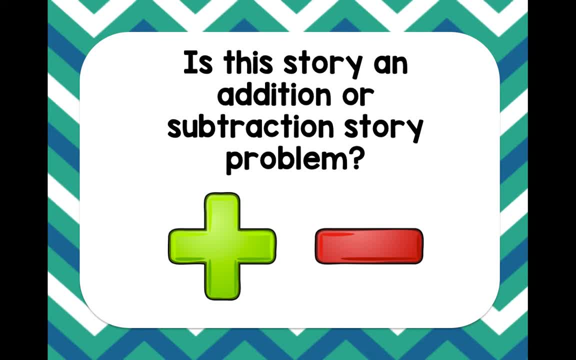 Is this story an addition or a subtraction story problem: Are we adding, with a plus sign, more bananas or are we subtracting with a minus sign, taking away some bananas? We're adding more bananas, Right, He's getting more from the zookeeper. 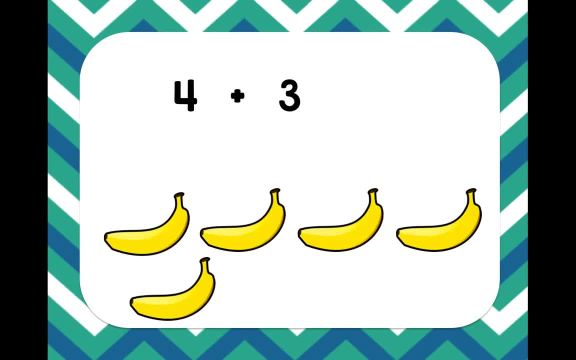 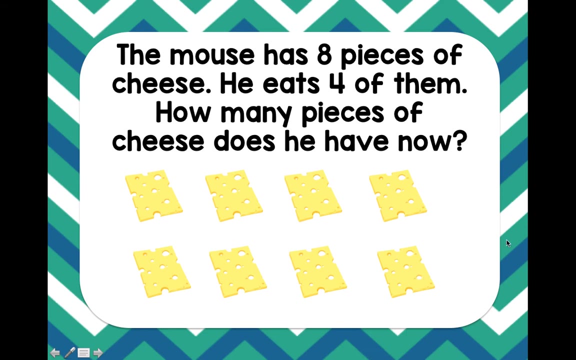 So he has four bananas plus three more bananas. One, two, three equals seven bananas. One, two, three, four, five, six, seven. Okay, The mouse has eight pieces of cheese. He eats four of them. How many pieces of cheese does he have now?